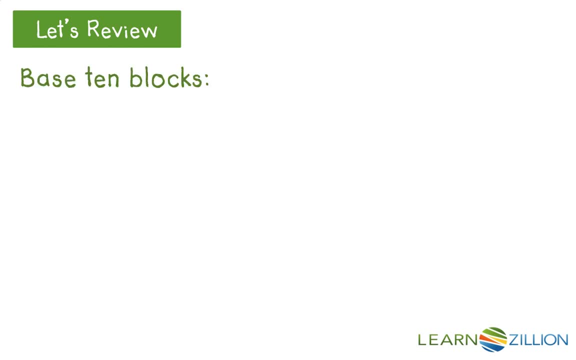 place stands for 3.. Here are the base 10 blocks we'll be using: One cube counts as 1, one ten long counts as 10, and one hundred flat counts as 100.. When I subtract really large numbers like this one, 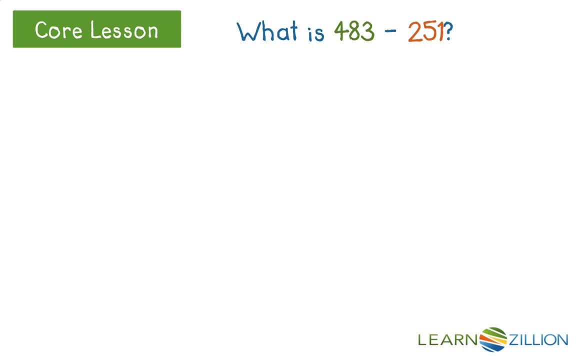 483 minus 251,. I like to line my numbers up in a hundreds, tens and ones chart so that I can see which base 10 blocks I'll have to draw out and how many I'll have to take away. So 483 minus 251.. We're going to use this, this chart. that's a. 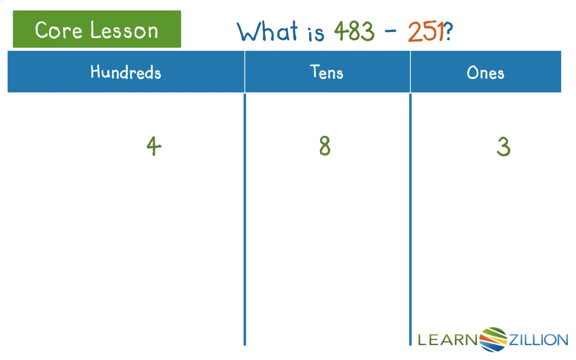 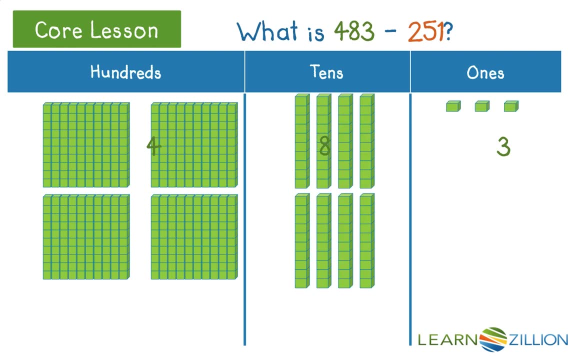 little bit bigger to fit all of our base, 10 blocks in. So first I start with 483.. I'll put out four hundredths, eight tens and three ones. I'm taking away 251.. So I'm taking away two hundredths, which leaves me with two hundredths. I'm taking away five tens. 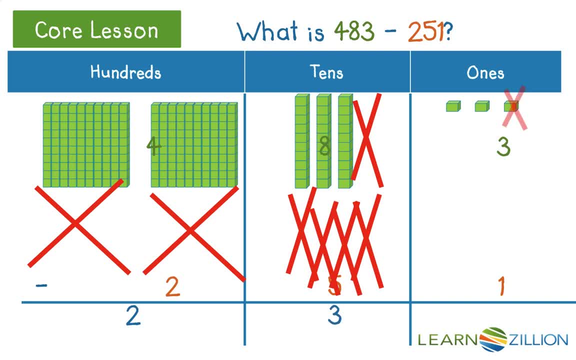 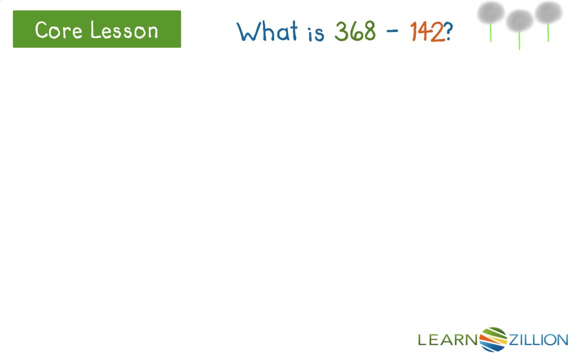 which leaves me with three tens, and I'm taking away one, one which leaves me with two ones. So 483 minus 251 equals 232.. Now remember, at the beginning we wanted to find out how many dandelions would be left if there were 368 in a field and 142 blew away. So we'll start with. 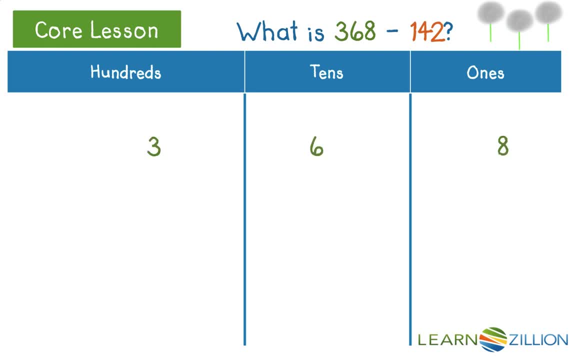 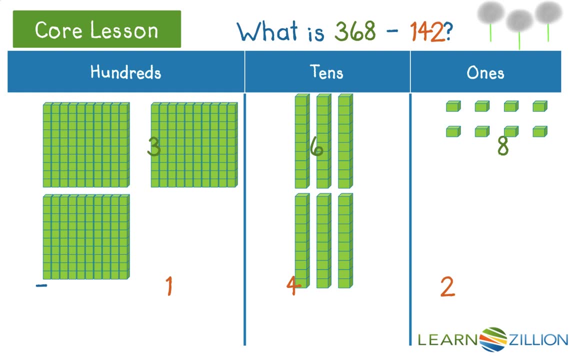 our hundreds, tens and ones chart, We have 368 to start, so three hundredths, six tens and eight ones, And we're taking away 142.. So we're taking away 100, which leaves us with two hundredths. We're taking away four tens, which leaves us with two tens, and we're taking away. 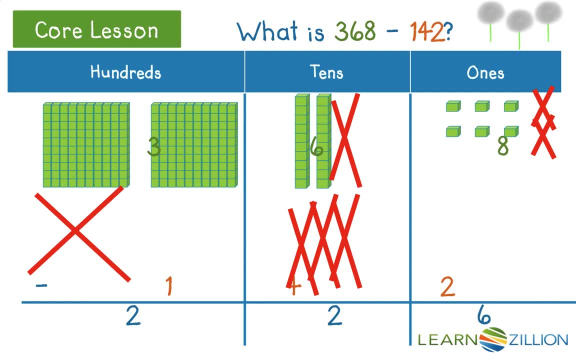 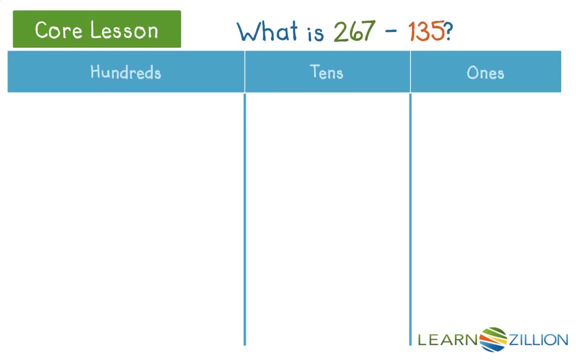 two ones, which leaves us with six ones. So if 142 dandelions blew away, we would still be left with 226.. Let's look at one more example. So we have 267 minus 135.. So I'm going to start the same way, putting out 200, two hundredths, six tens and seven ones.